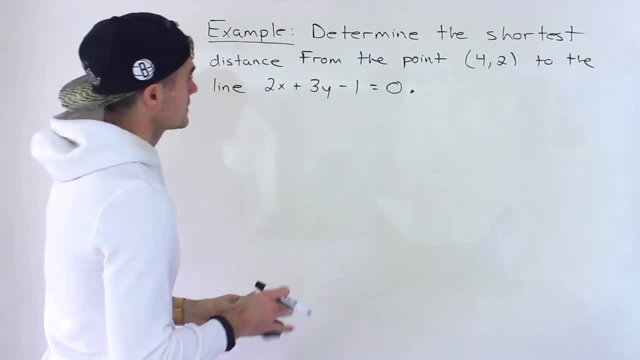 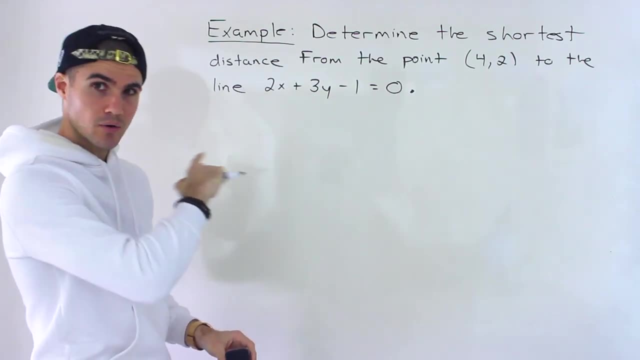 watched that. So let's go here. so notice that we're given this line here. notice that the line is actually in standard form, which is nice, because when we use that formula, the line has to be in standard form. so we're not going to have to rearrange this, but we are going to have to. 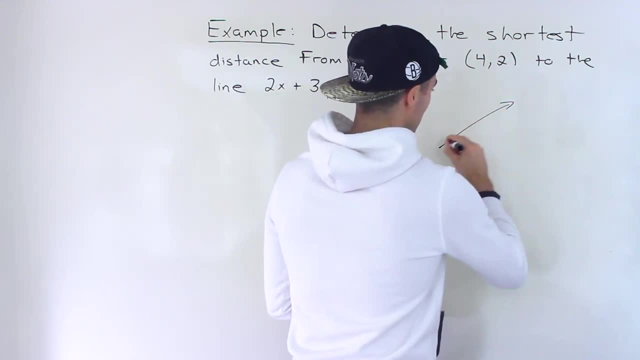 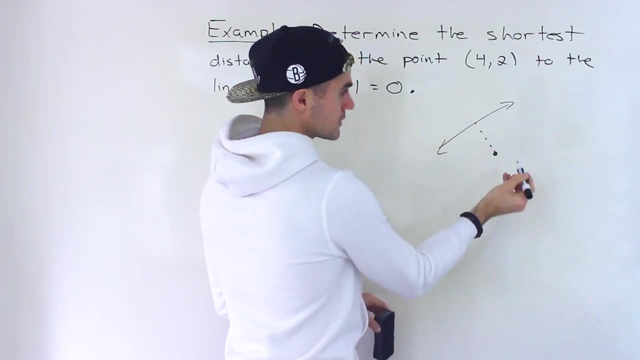 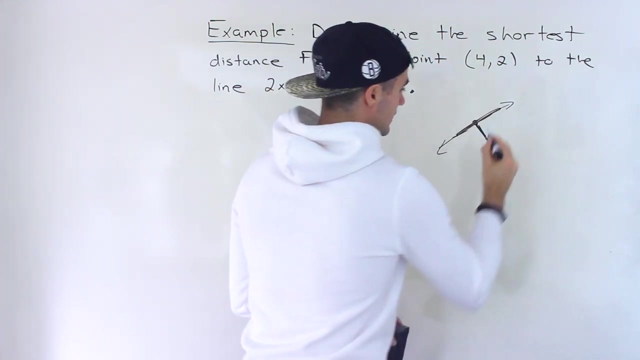 use that in order to get all of the lines of the curve here, because, if you remember, what's happening is just, in general, if we have a line, we have a point to find the shortest distance. it's going to be the perpendicular distance. we're going to have to find the point of intersection between this. 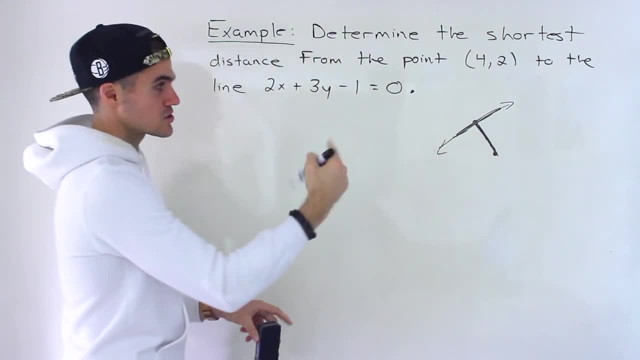 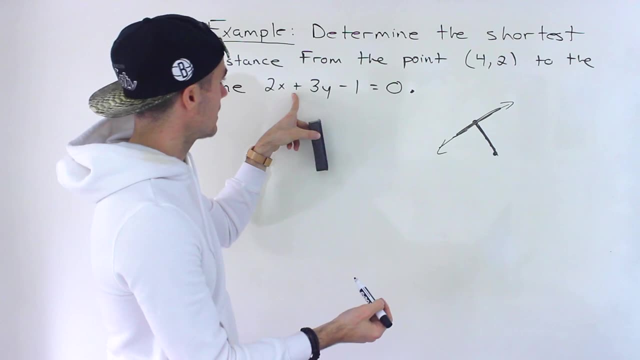 line and this line and to do that, we're going to have to get the equation of this line, which means we're going to have to get the slope of it, which means we're going to have to get the slope of this line over here that we're given. 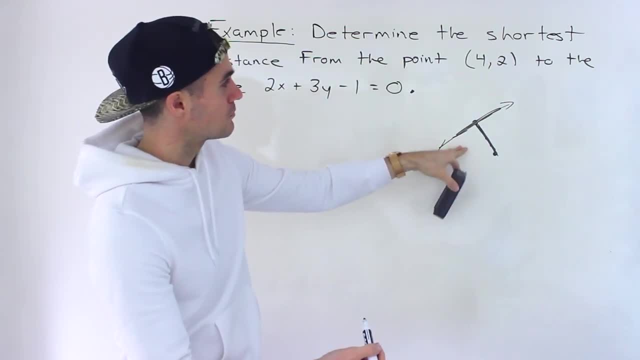 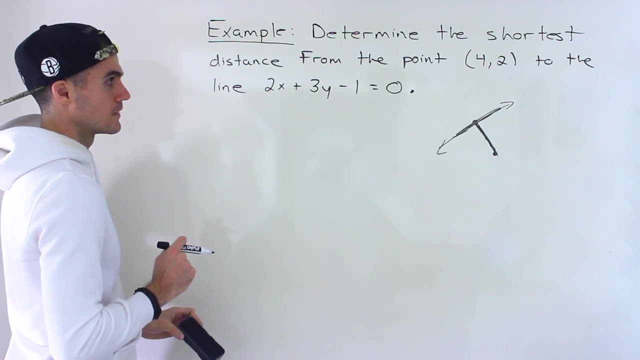 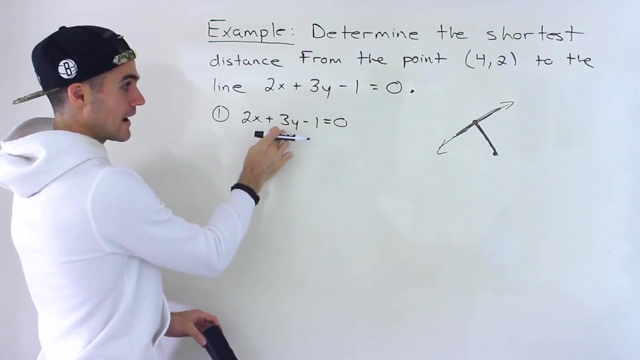 a negative slope. so this is not an accurate representation of this scenario, but just kind of giving you the general overview of what we're going to be doing. so let's first take this line here and change it to: y equals mx plus b4. so what we do then is we have to isolate for this y here. 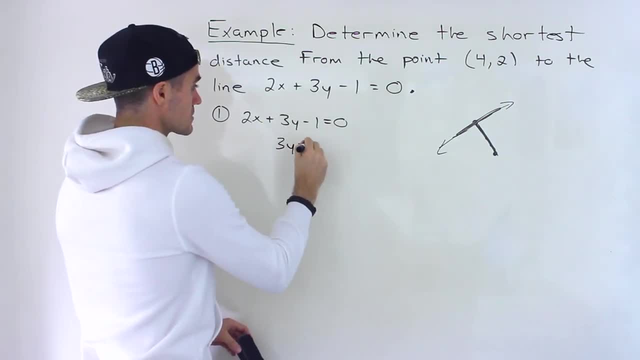 so let's bring the 2x over, bring the negative 1 over, so we'd have y equals or 3y equals negative 2x plus 1. we could divide everything by 3 and we'd end up with y equaling negative 2 over 3x. 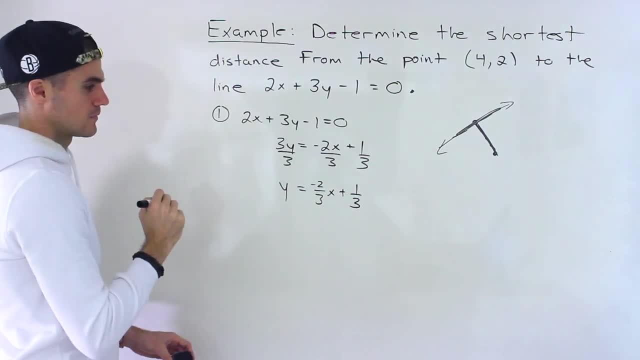 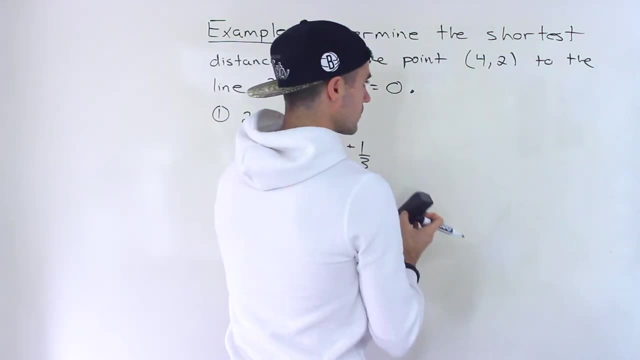 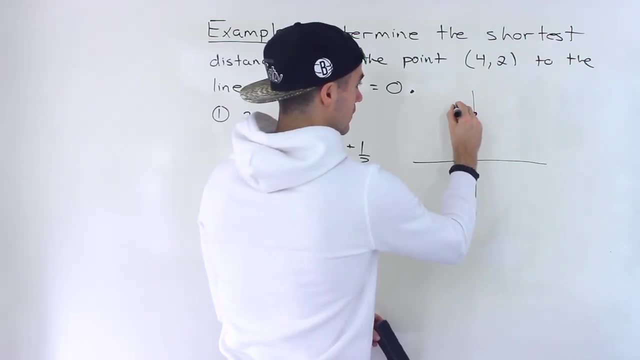 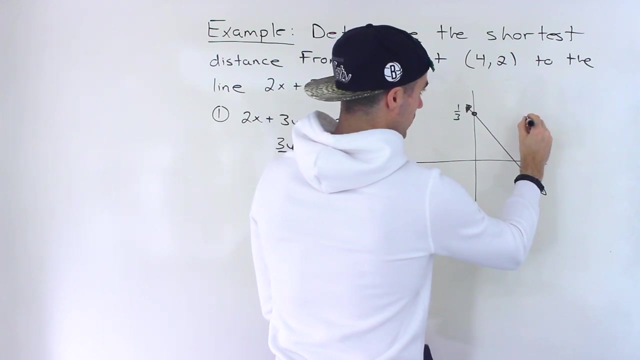 the b value. so that's going to be over here. and then notice it has a negative slope. okay, so it's going to look something like that over here. and then 4 and 2. it's going to be like somewhere. let's say i'll just put it here. oh no, 2 is going to be above the 3, so let's put it like up here again. 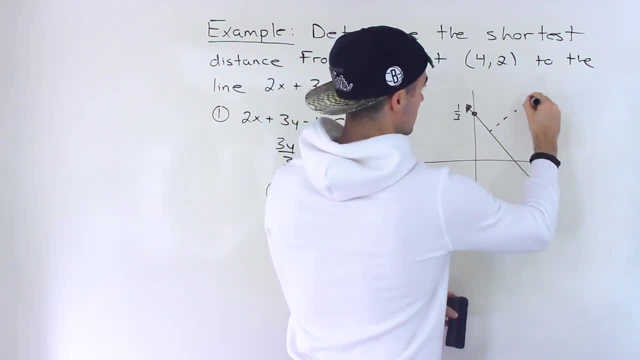 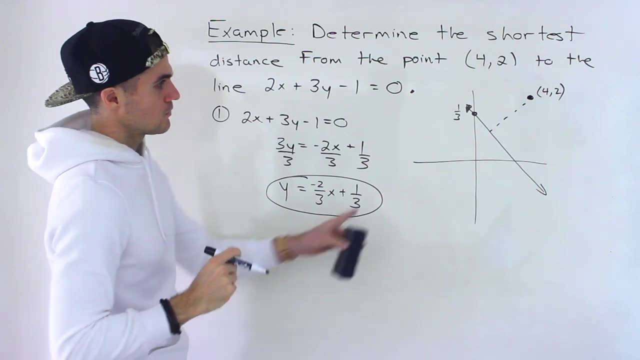 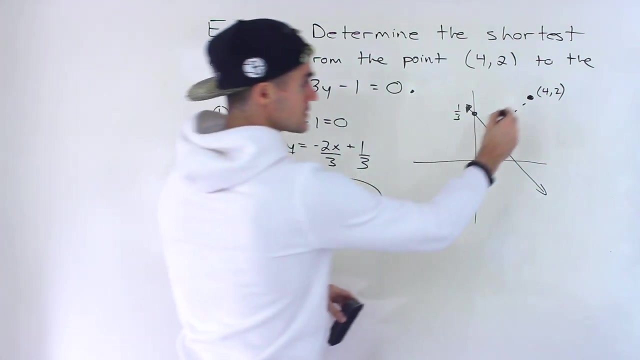 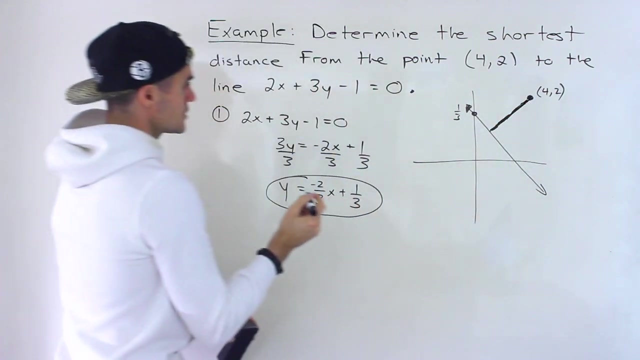 this is not to scale. i'm just kind of showing you roughly what's happening. all right, so this line over here it's this line or this line, both of them are the same thing. and then 4 and 2 is up here. we got to find this distance over here. so notice that this line here it has a slope. this line, right that? 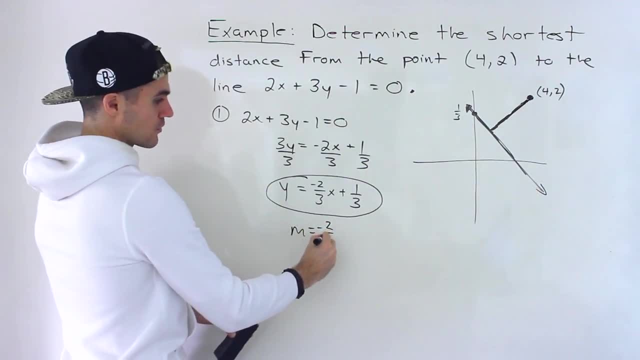 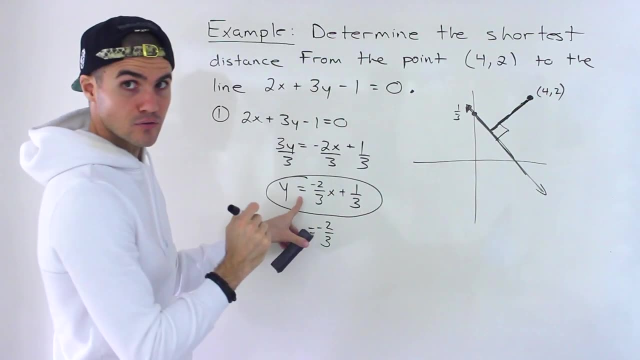 we're working on and then we're going to find this distance over here and then we're going to find this distance over here that we're working with. it has a slope of negative 2 over 3, so we need the slope of this line and because that line is perpendicular to this line over here, the slope is. 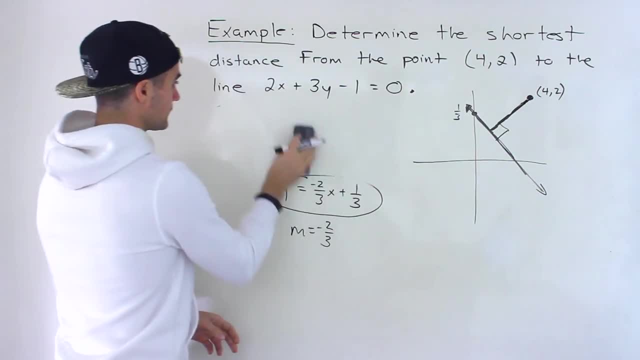 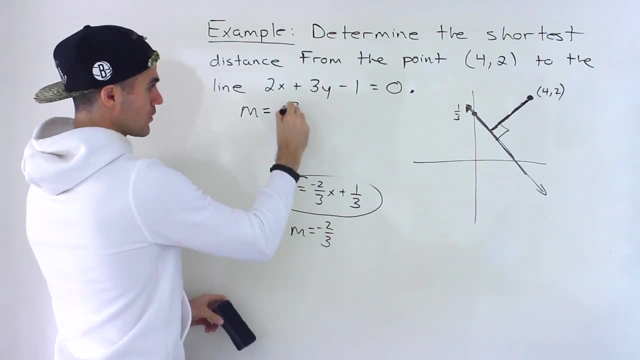 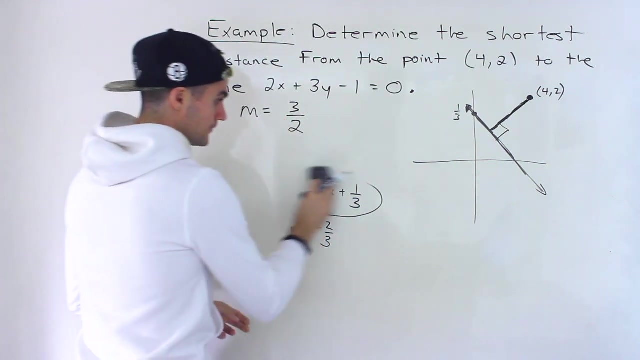 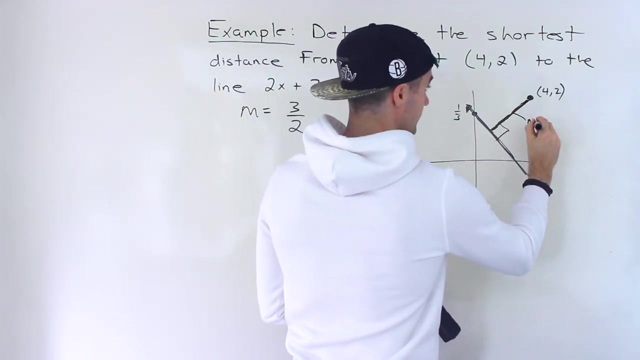 going to be the negative reciprocal of that. so the slope of this second line here is going to be this: flipped over 3 over 2, and then the sign change. so notice, this is negative, this is going to be positive. and so now what we can do. we have the slope of this line. It's 3 over 2.. And we have a point on that line. 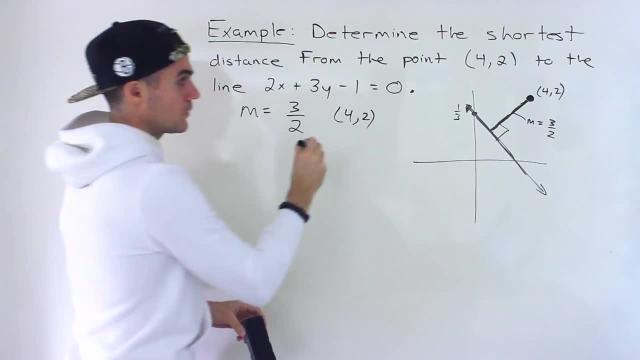 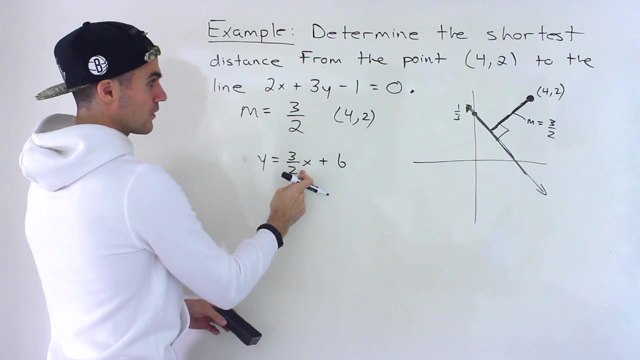 So we have a slope, We have a point, We can find the equation of the line now. So we'll have y equals, or sorry, y equals 3 over 2, x plus b. To solve for this b value, we could plug in 4 for x. 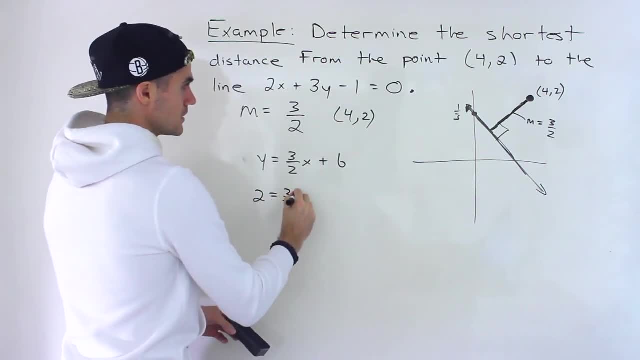 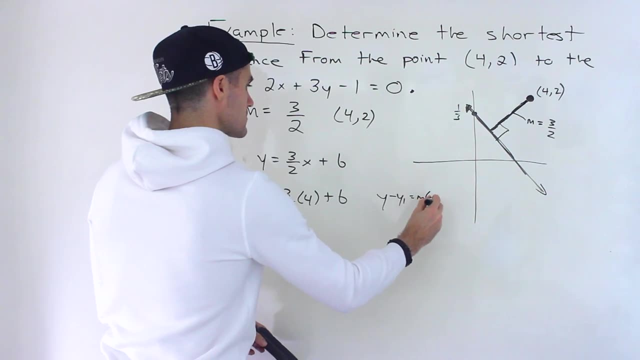 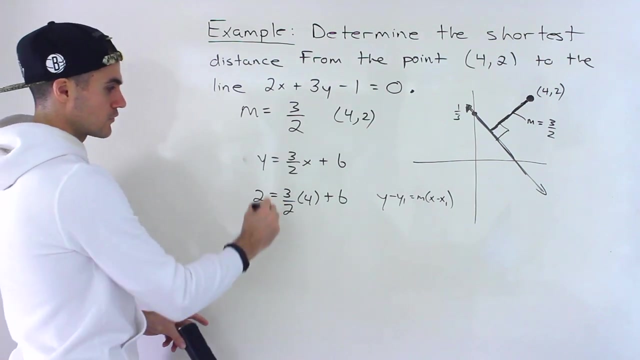 We could plug in 2 for y. At this point you may also be using that other formula where we have y minus y1 equals nx minus x1.. To find the b value, just make sure you're getting the exact same equation at the end that I'm going to get over here. So we'll have 2, 3 over 2 times 4.. 2 goes. 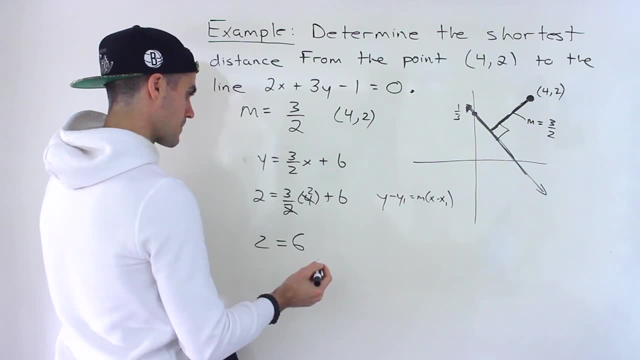 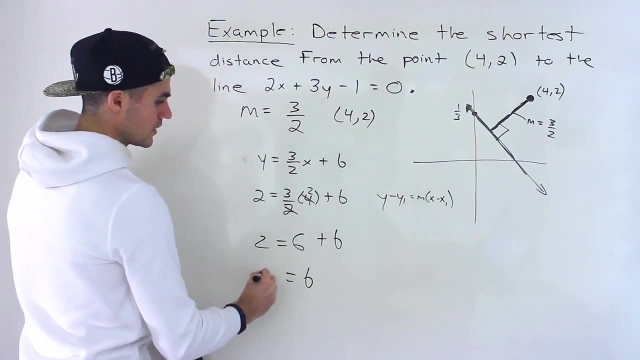 into 4 twice, So this would end up equaling 6.. All right, Yeah, 6.. And then we got plus b, So b would equal negative 4.. When we bring the 6 over, 2 minus 6: 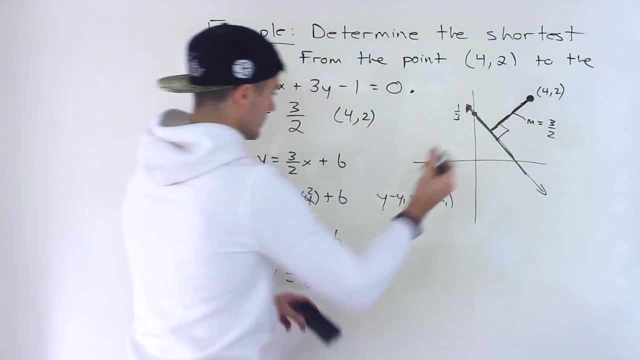 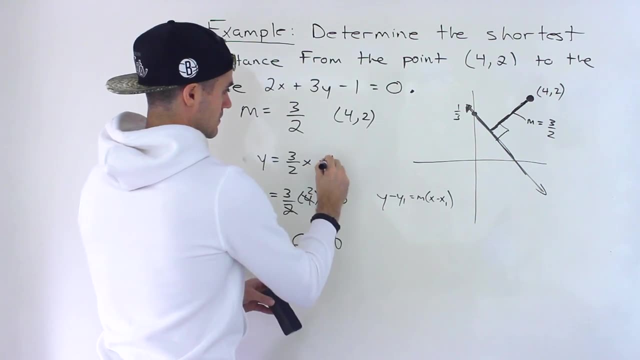 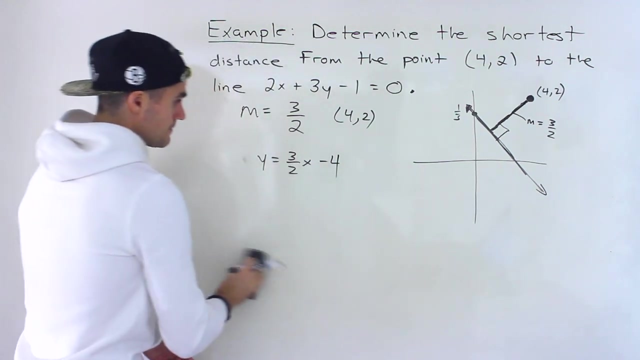 is negative 4.. So this line here, we got the equation of it. We got 3 over 2 x minus 4.. Like that. So now, what's the next step? Well, we got the equation of this line, We got the equation of: 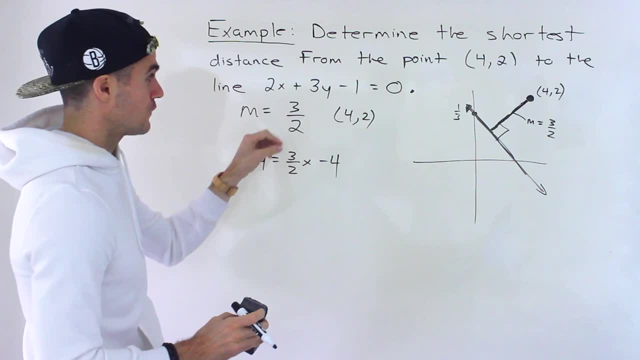 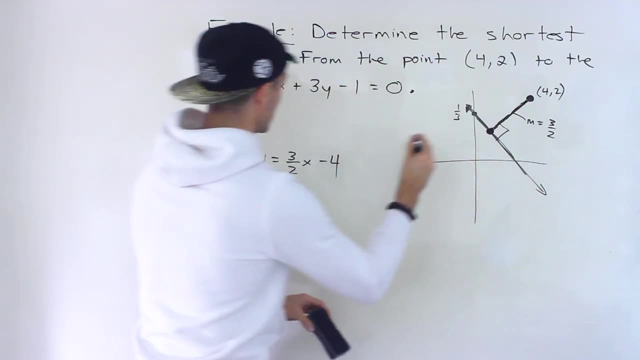 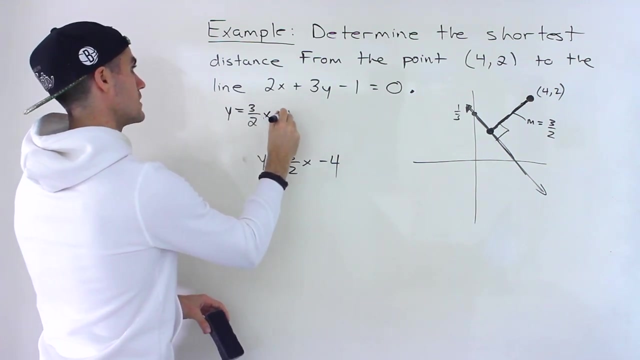 This line, And now we have to find the point of intersection between them. All right, We got to find this point over here. So we got y equals 3 over 2, x minus 4. Like that, And so from here. 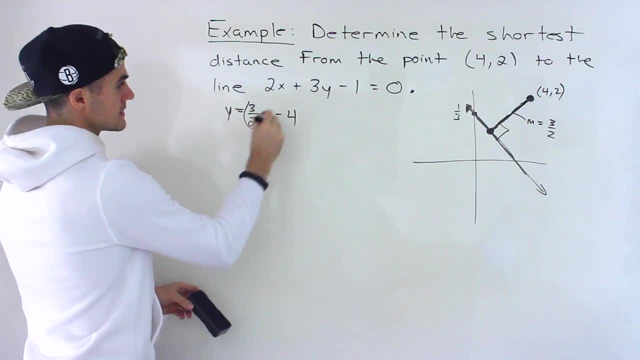 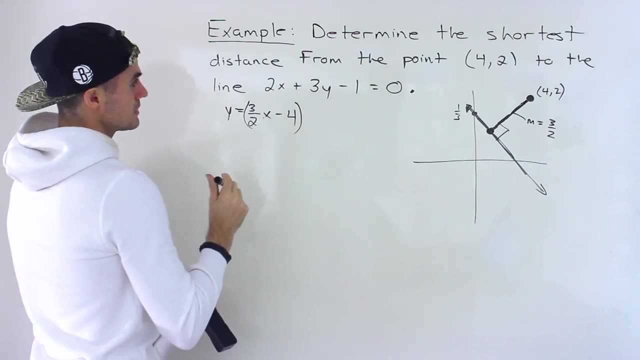 I feel like the y is already isolated, right, So let's just take this, plug it in here, Or actually, you know what? Let's actually I was going to say we change this to y equals mx plus b format. We could just make both of those. 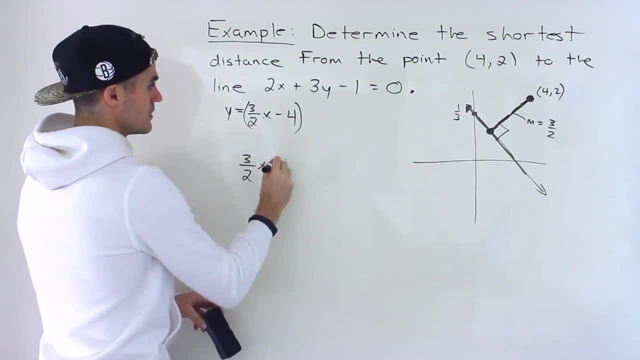 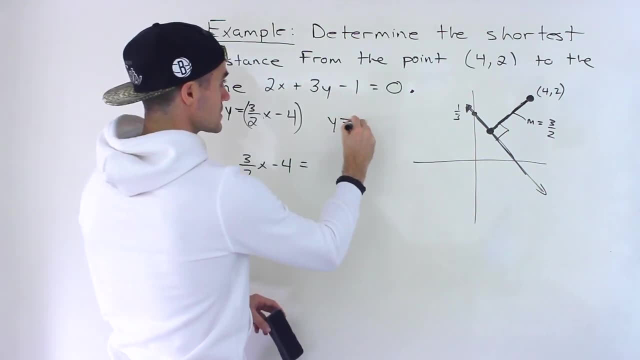 lines equal. Yeah, Let's just do that. So we'll have 3 over 2 x minus 4 equals. Remember this line here, this standard form line. I erased it, but it was negative: 2 over 3 x plus 1 over 3.. 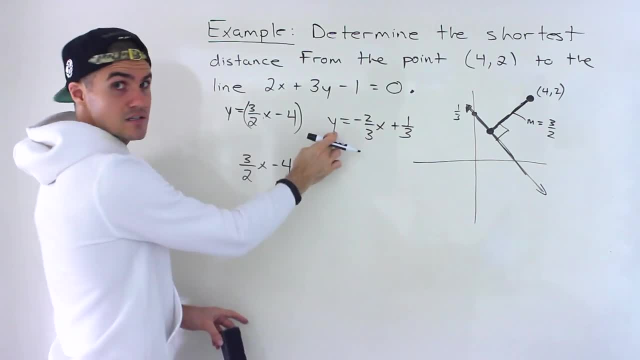 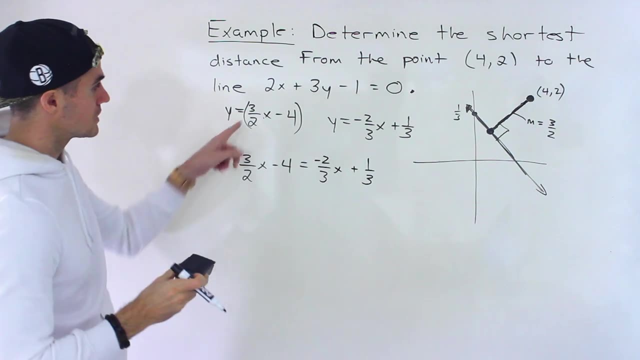 So we can let this equal that Plug in this for that y value. So this would be negative 2 over 3, x plus 1 over 3.. Whichever way you do it, you could take this, you could plug it in for this y, So you'd have 3 bracket all of that. 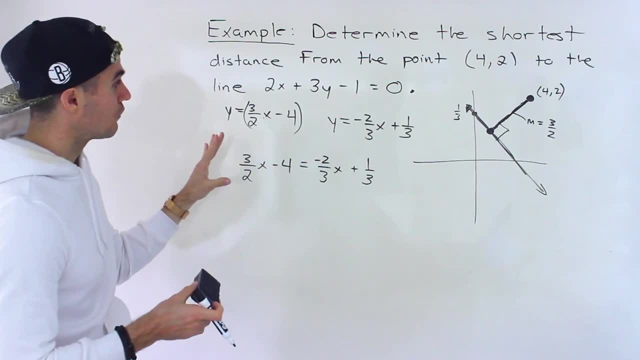 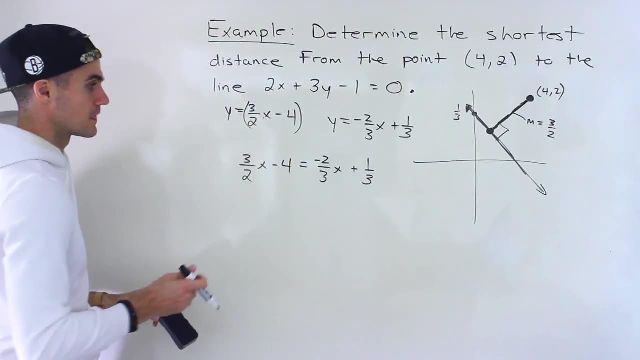 And then you could solve for x Many different ways. you could solve for x and y with these two equations. Just whichever way you do it, make sure you're getting the same point of intersection that I'm going to get. So bring all of the x values to one side. 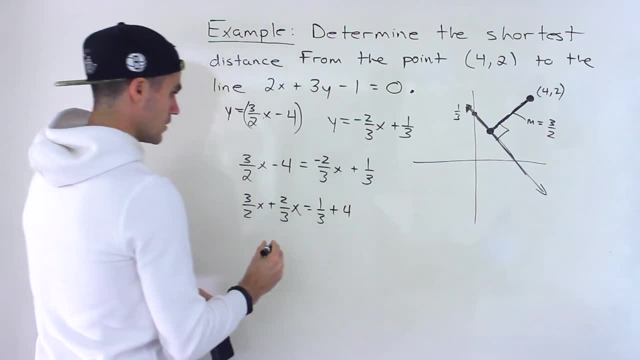 And then I'm going to bring the negative 4 over, So we'll have- Let's do this on the side- 3 over 2 plus 2 over 3.. Lowest common denominator between 2 and 3 is 6.. Multiply this by 3,. multiply this by. 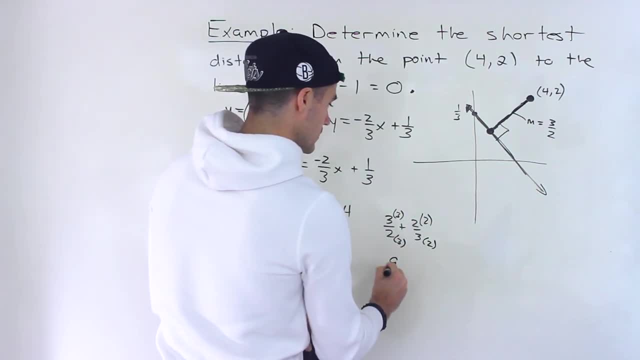 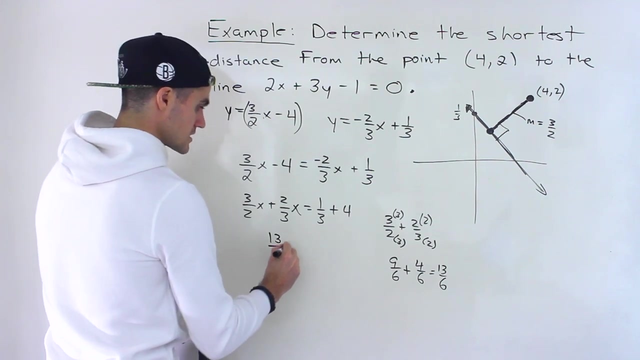 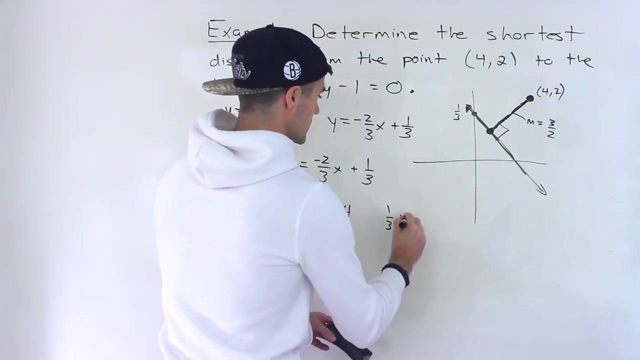 3,. multiply this by 2, multiply this by 2.. So we'd have 9 over 6 plus 4 over 6,, which would give us 13 over 6.. So we'd have 13.. 13 over 6x equals 1 over 3 plus 4 over 1.. Lowest common denominator between 3 and 1 is 3.. So multiply. 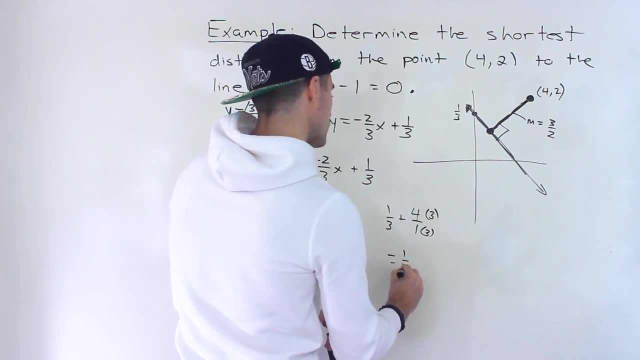 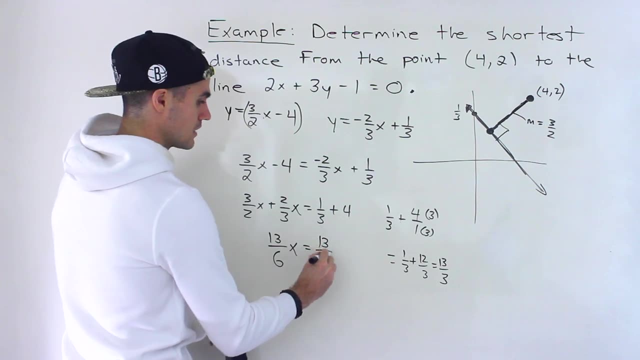 this by 3, multiply this by 3.. We'd end up with 1 over 3 plus 12 over 3, which would give us 13 over 3, like that. So this would be 13 over 3.. 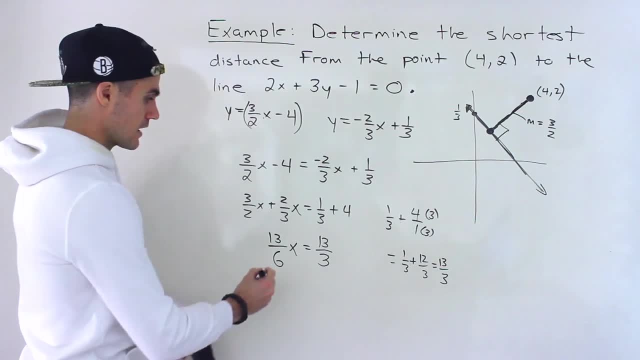 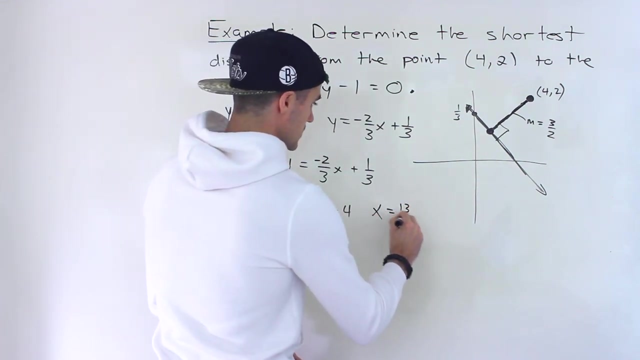 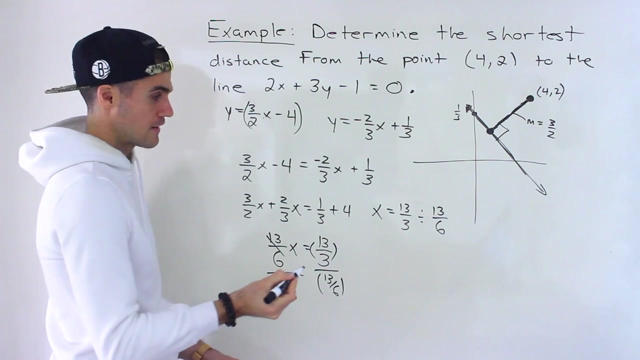 So from here, what we would do is to isolate for this x, we would divide both sides by 13 over 6.. So these cancel x would equal 13 over 3, divided by 13 over 6, right, This fraction divided by that. 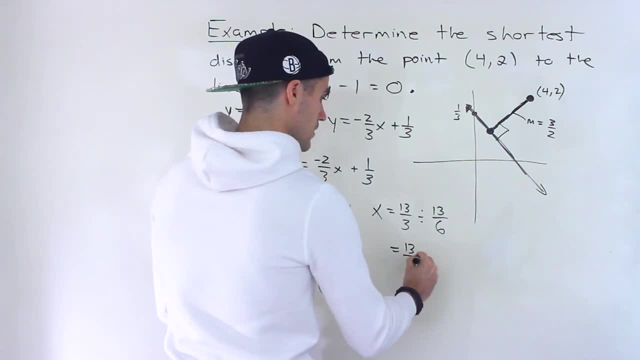 fraction which would give us 13 over 3, multiplied by 6 over 3.. So we'd have 13 over 6 plus 4 over 3.. So we'd have 13 over 6 plus 4 over 13.. We would flip this fraction. Notice the 13s, cancel out. 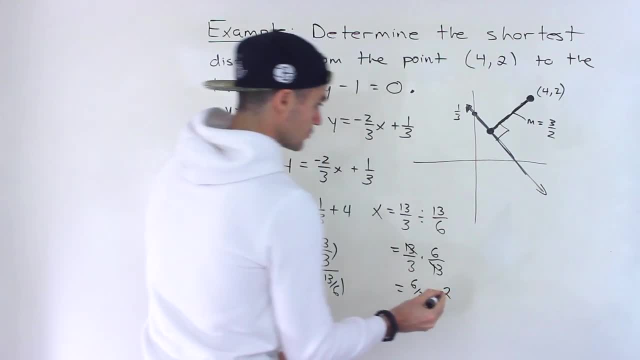 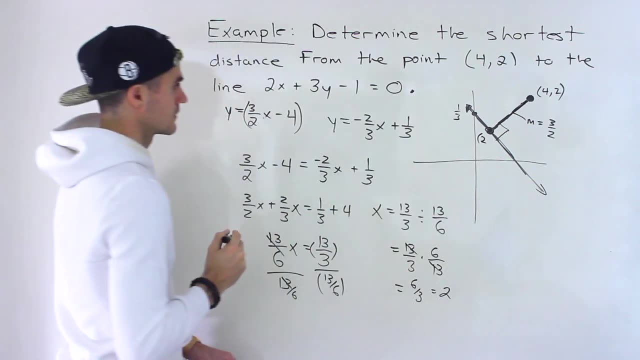 And then we'd have 6 over 3,, which would just give us 2.. So the x value of this point is 2, like that, And now we just have to solve for the y value, So we could plug it into. 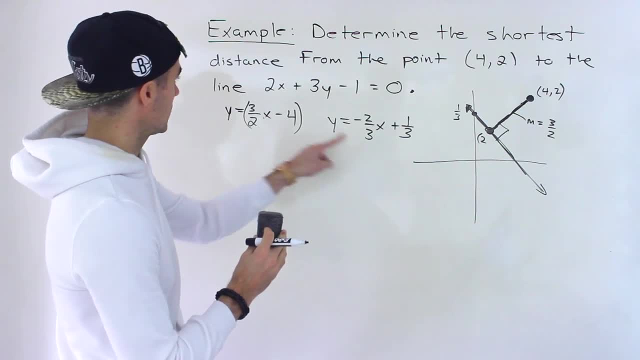 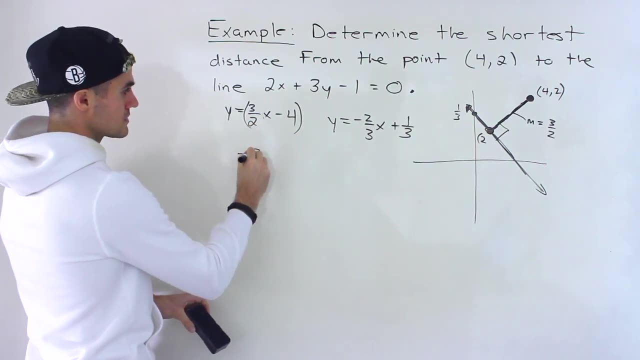 We could plug in that x value of 2, either here or here. I'm going to plug it in here because notice, Notice that if we plug in 2 here, these 2s would cancel out right. So we wouldn't have. 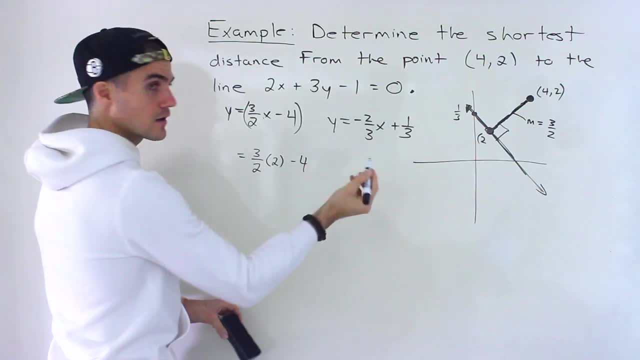 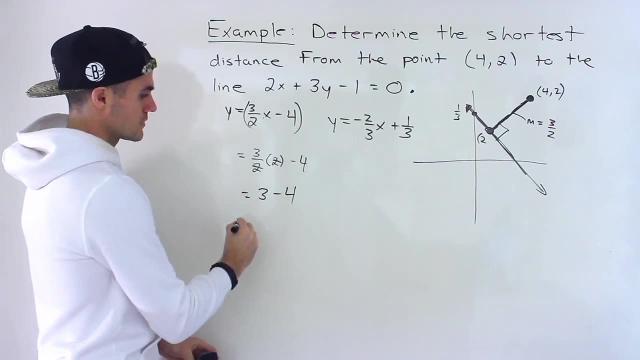 to work with fractions then. But again, if you want to plug it in here, you'll still get that same y value. So this would be the 2s. cancel out And notice we'd have 3 minus 4 left, which would give us negative 1.. So the y value would be negative 1.. 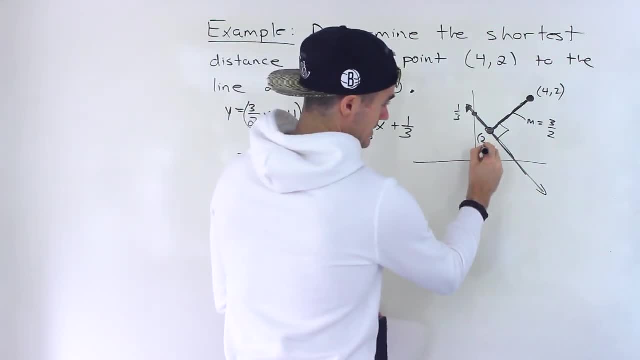 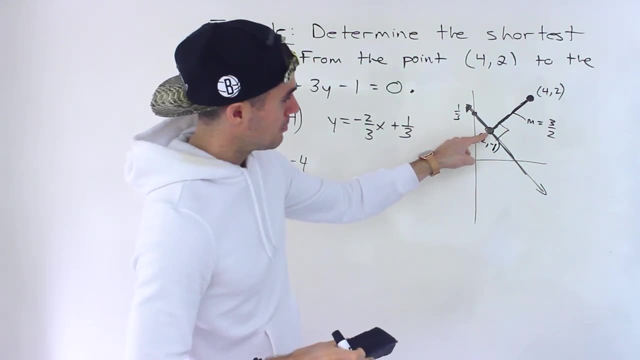 And then notice that at this point this ends up being negative 1.. But what's happening here? Well, this point here that I drew it's actually incorrect, right, Because this point here, if this is the Cartesian plane, this point would have a positive y value. 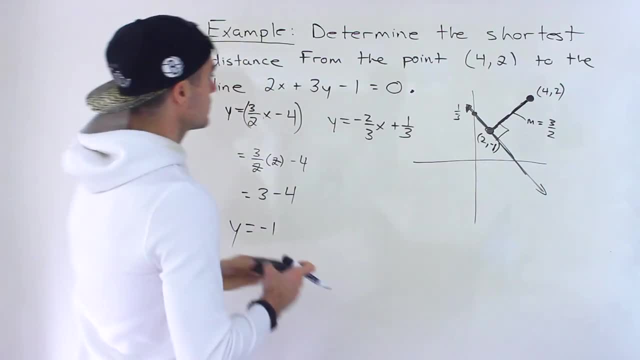 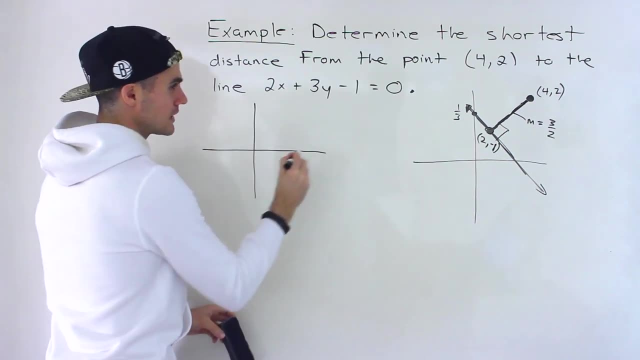 but it has a negative y value. okay, So I made a rough drawing there. but this is an example of where, even if you make a rough drawing, sometimes you're going to get results where you have to adjust the drawing. So this is an example of where, even if you make a rough drawing, sometimes you're going to get results where you have to adjust the drawing. 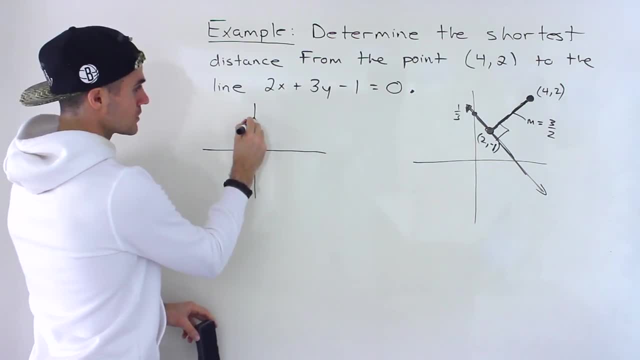 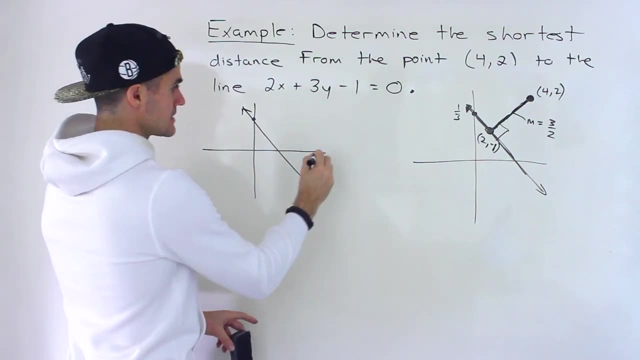 And so the way this actually looks like, if we go into more detail, now that we have more detail, what's happening is that this point 4 and 2, it's like way out here, okay, So if we find the perpendicular distance, it's actually going to be like let's anyway. 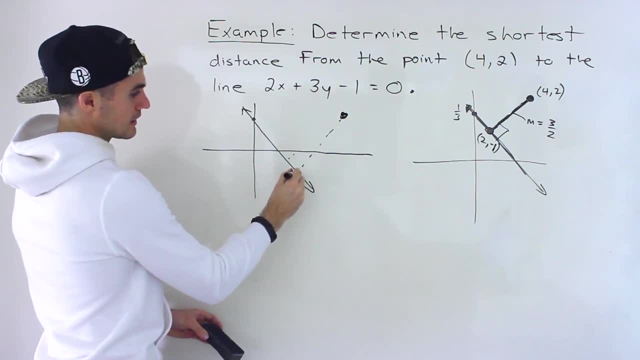 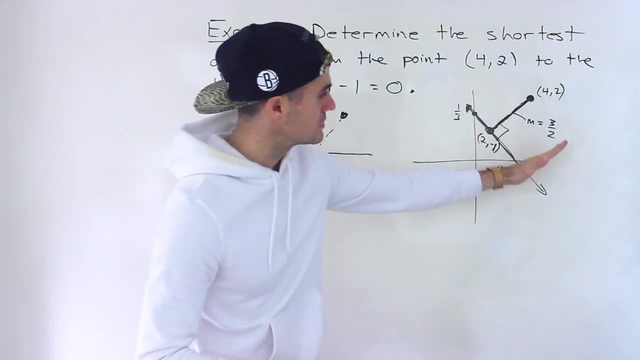 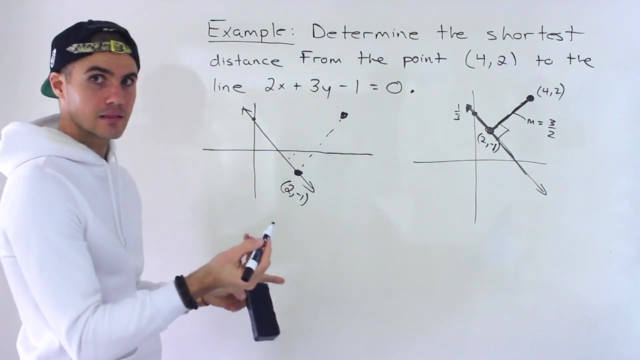 it looks something like that. So this point, this point of intersection, is actually going to be in this quadrant, right? So this could- should be sort of shifted downward, okay, And I didn't know that until we did a little bit of more. 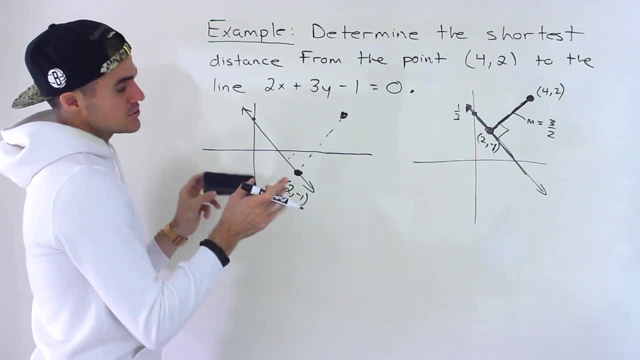 work For these kinds of questions, unless your teacher really wants you to graph it. you don't even have to graph it on a Cartesian plane. You can just draw a line and then draw a point just to have like a video or a drawing or something like that. 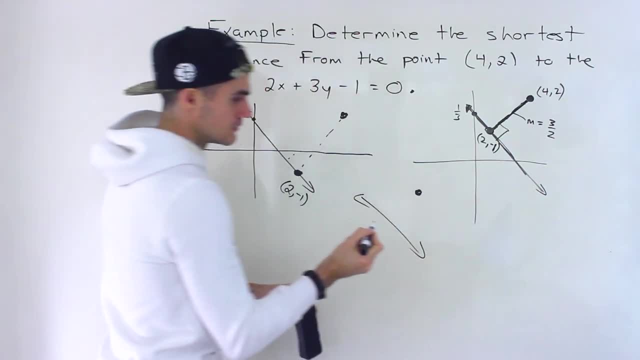 you don't even have to graph it on a Cartesian plane, You could just draw a line and then draw a point, just to have, like a video or something like that, a visual rough reference of what we're doing. And then, when we got this point to a negative one, 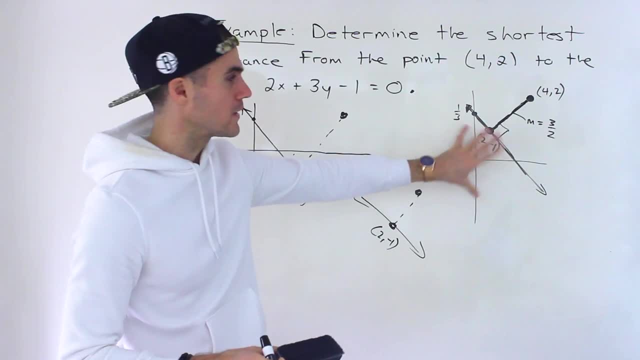 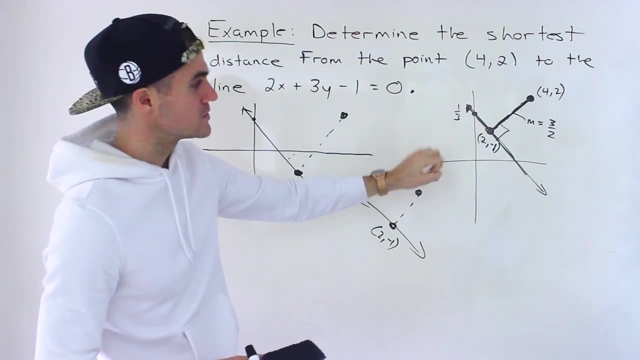 we don't necessarily have to go and go into details and waste time on that, but your teacher may expect you to know how to graph it or to graph it, and if so, then you got to take more time, go into more detail, a lot more time than I did, right, Because notice that I didn't take the time. 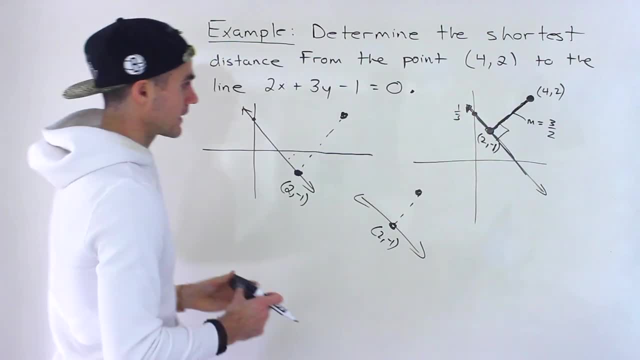 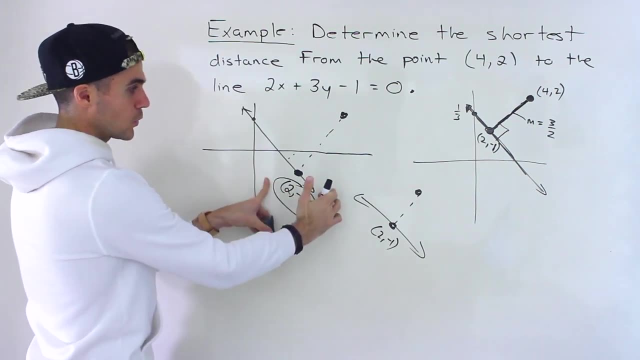 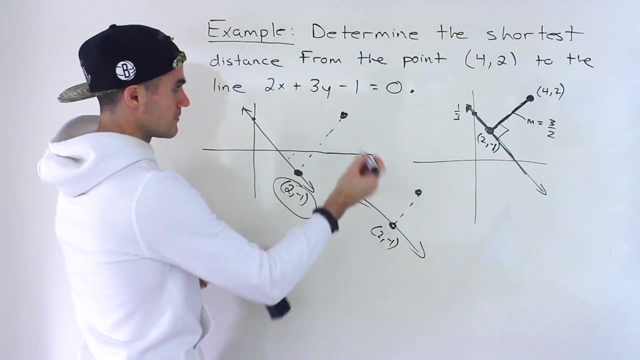 to go into detail here, and so this drawing was incorrect. The drawing should be something like this: approximately: Basically, that point of intersection is going to be in this quadrant versus that one. okay, But same process is still applying. We're still finding the point of 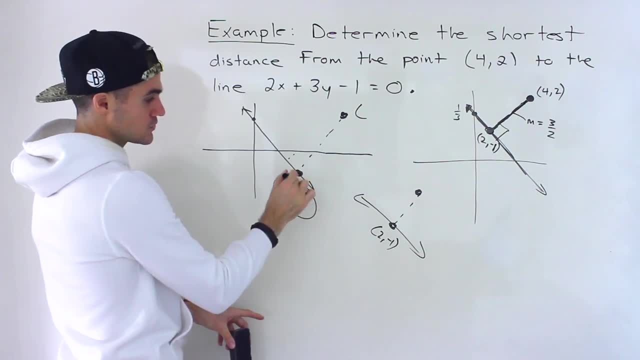 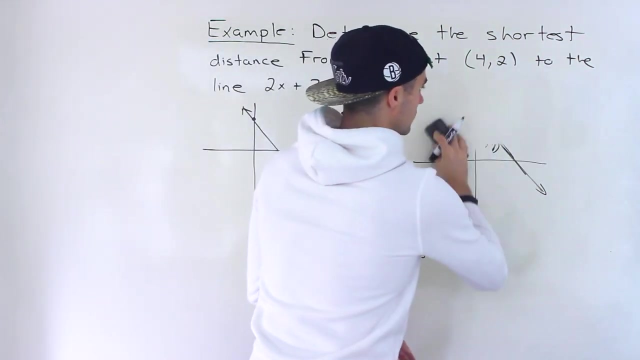 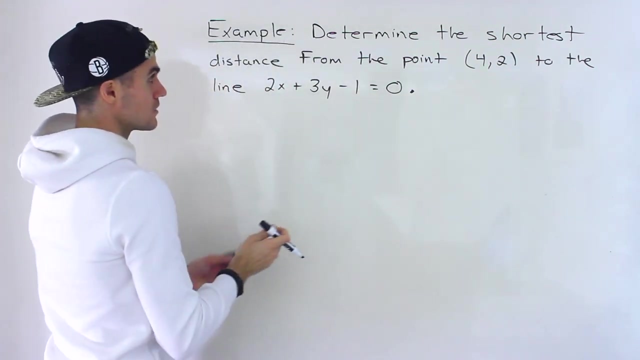 intersection between two or the distance, rather between two and negative one, and then that point, Four and two, right. And if we had the general drawing here, two negative one, four and two. So to do that we got to use the length formula. So let's write two negative one here. So I'll let 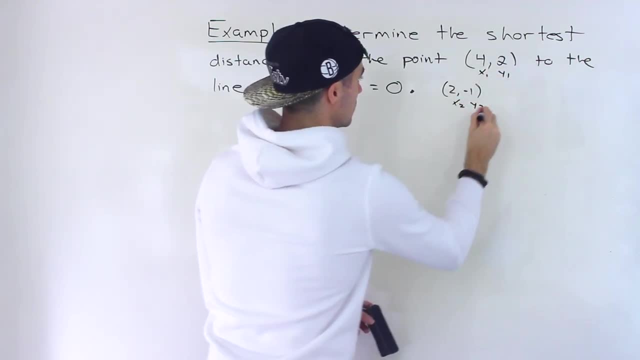 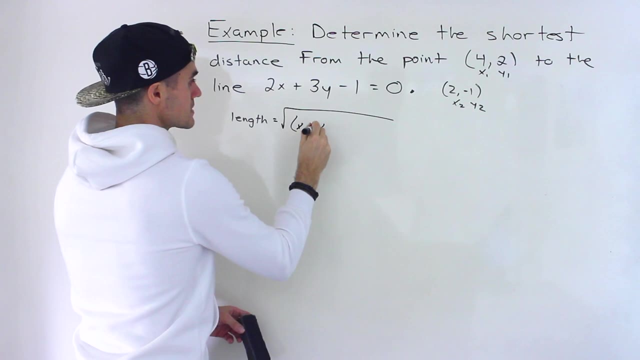 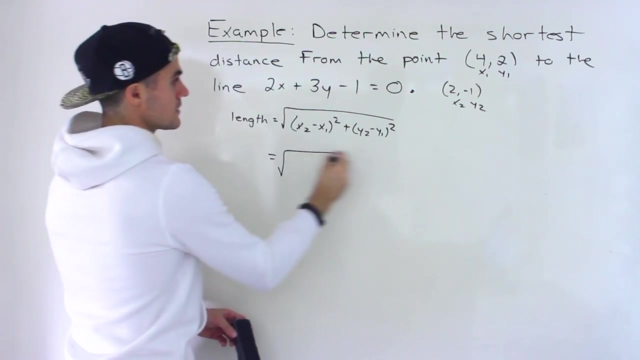 this be x one, y one, x two, y two. So we know the length or the distance between two points is equal to the square root of x two minus x one squared, plus y two minus y one squared. Okay, so here we got x two. 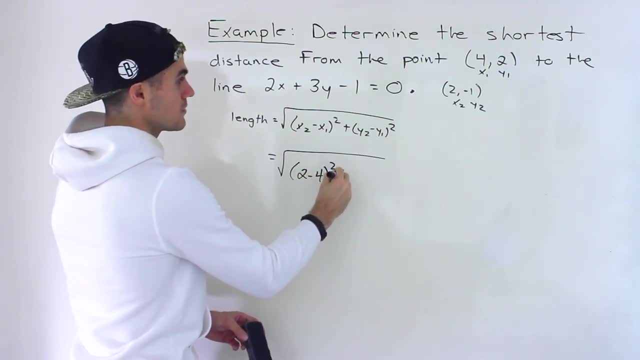 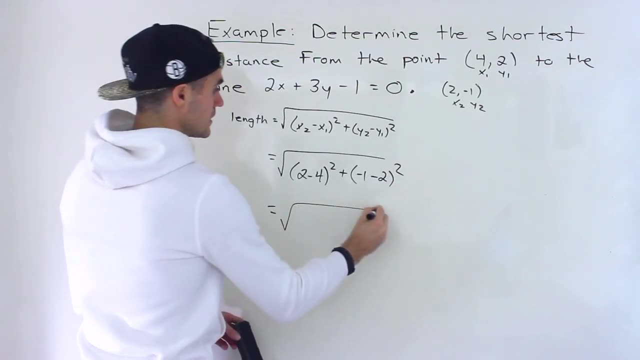 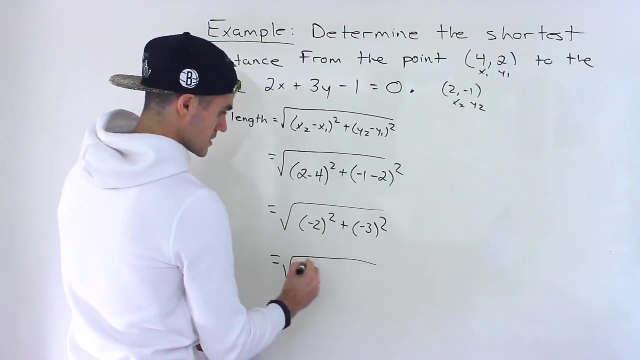 which is two minus x, one which is four squared plus y two. negative one minus y, one squared like that. So this would end up equaling negative two to the power two plus negative three to the power two, which would give us four plus nine. 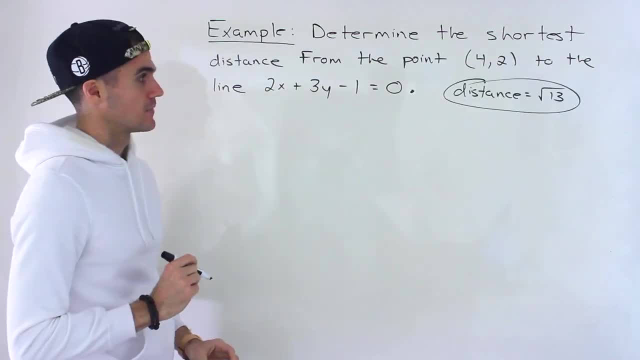 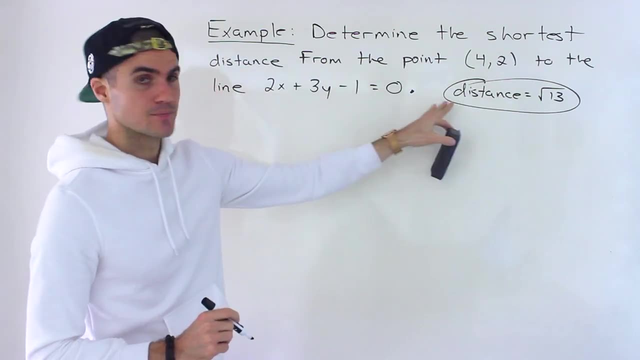 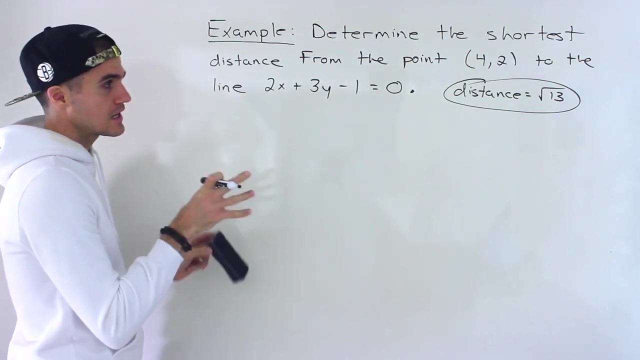 which would give us root 13.. So that ends up being the final answer. That's the shortest distance between this point and this line, right Square root of 13.. So now what we can do is use that formula see if it matches up. So if you remember the shortest distance between a line in standard, 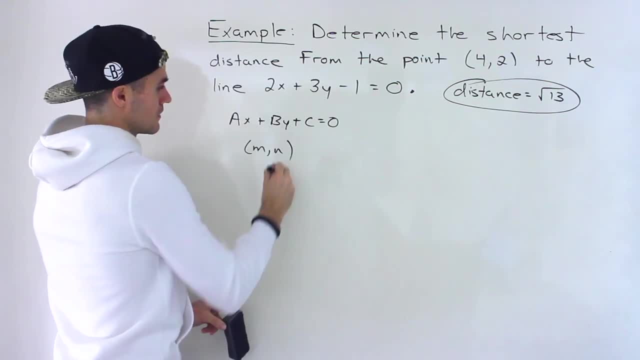 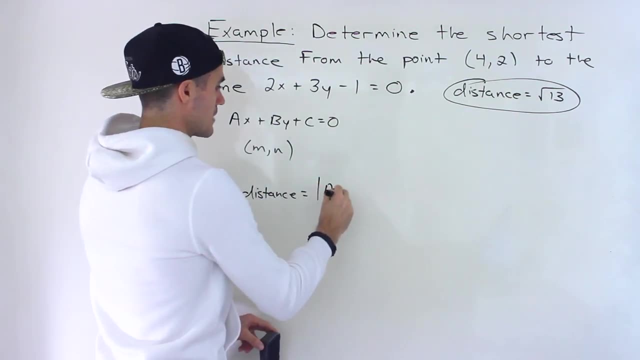 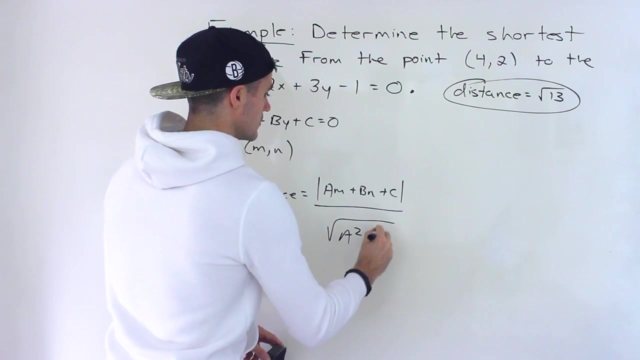 form and a point, m and n, the distance between those is going to equal the absolute value of a, m plus b, m plus c, all over the square root of a squared plus b squared. And so notice again, as I mentioned at the beginning, it's nice that. 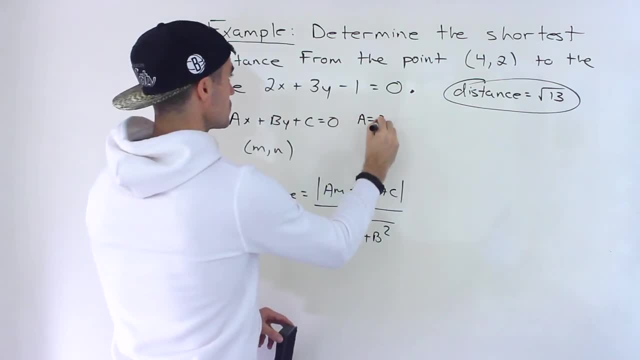 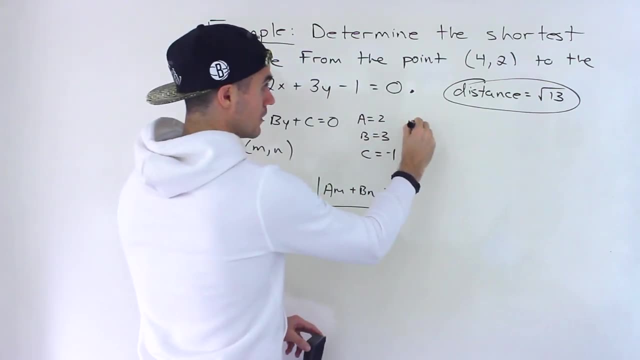 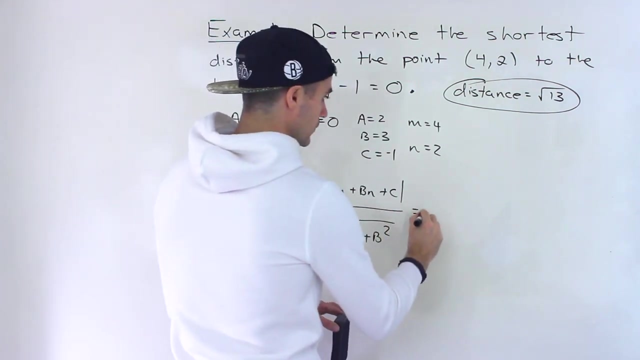 this line. it's already in standard form, So notice: the a value is two, the b value is three, the c value is negative one, the m value is four, the n value is two. So what happens when we plug everything in? Well, we'd have the square root of the a value. 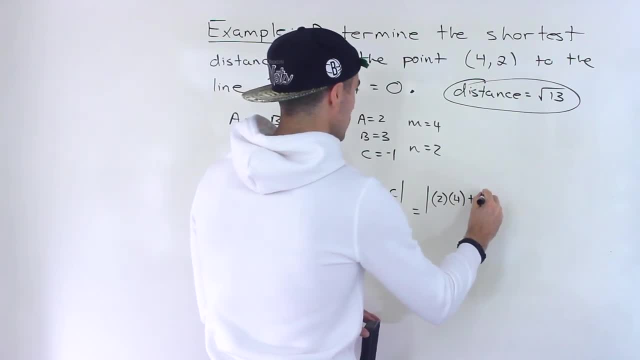 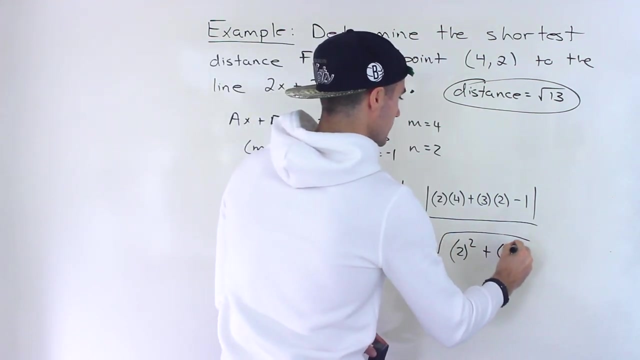 which is two times the m value, four plus the b value, three times the n value of two minus one. for the c value all over, the square root of the a value is two and then the b value is three, like that. So what happens here is we'd end up equaling. 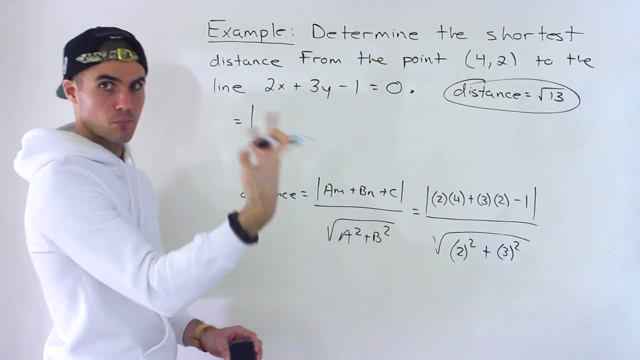 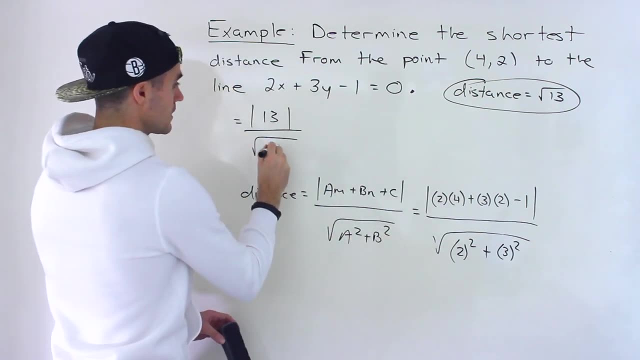 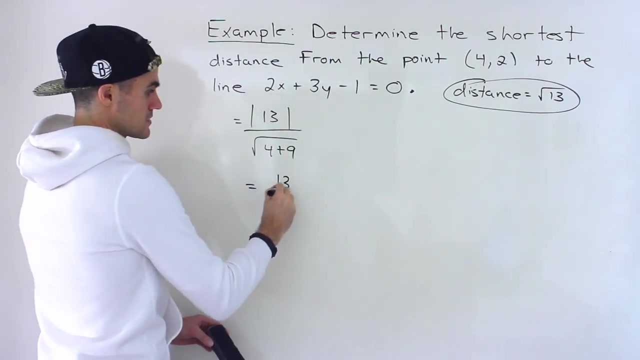 eight plus six, which is fourteen minus one, is thirteen, So we'd have the absolute value of 13 over the square root of four plus nine and we'd end up with the absolute value of thirteen is just a positive, so it stays as a positive, and then this would end up equaling the square root of. 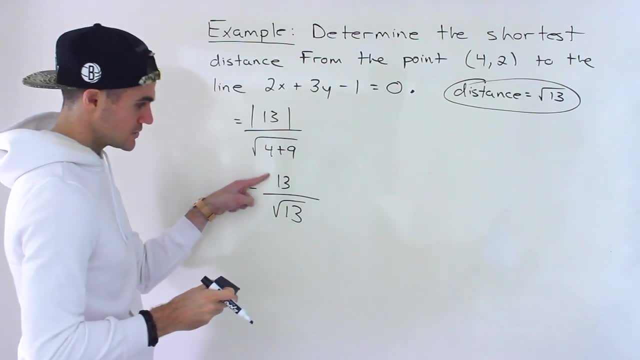 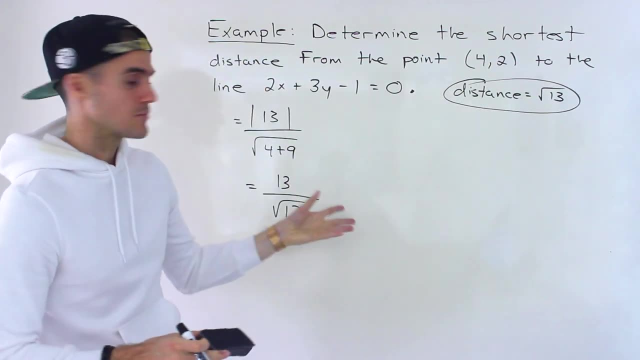 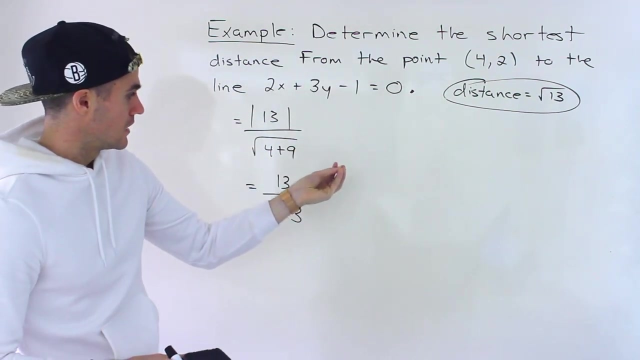 thirteen. So wait what's happening. We have thirteen over root 13,. and then we have root 13 here and you may think they're different. they're actually the same thing. if you take this, plug it into your calculator, take this, you'll get the exact same decimal. question is: how can we take? 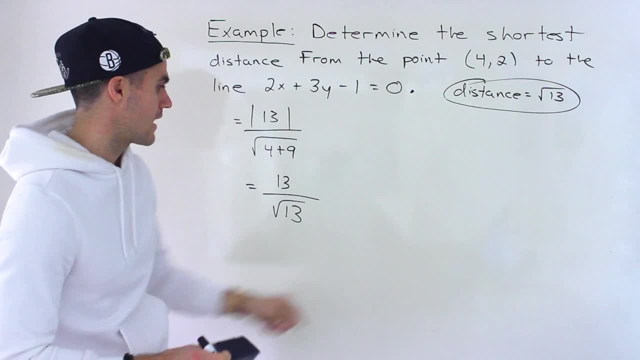 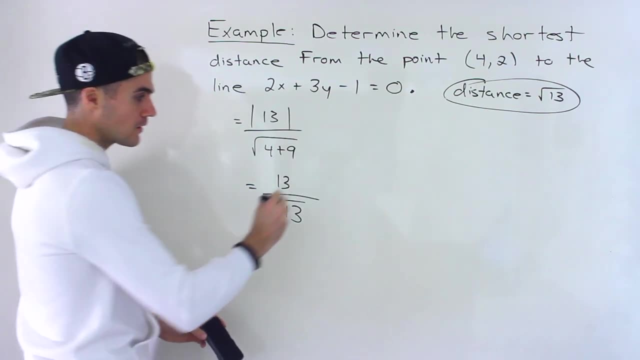 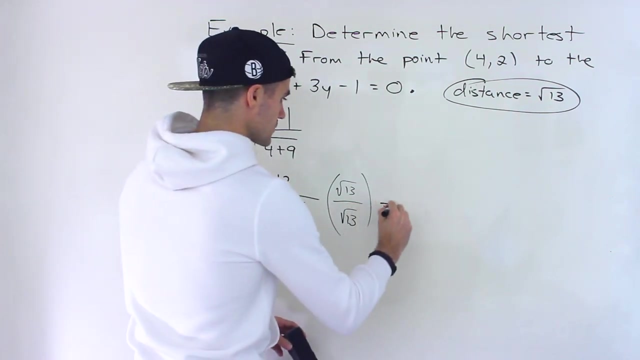 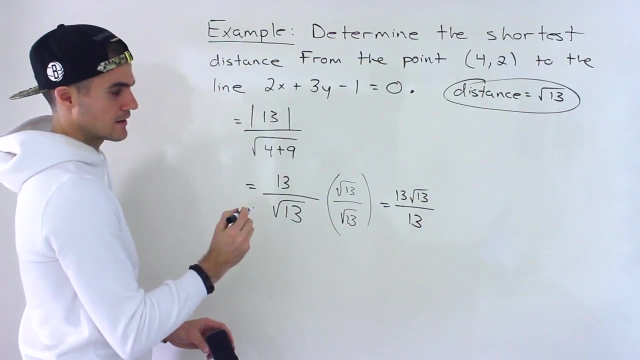 this and convert it to that. well, we can rationalize the denominator. i went through that in the example before. what we can do is we can multiply this by root 13 over root 13, which equals 3 root 13, and then root 13 times root 13 is 13, like that, and then notice the 13s would cancel out. 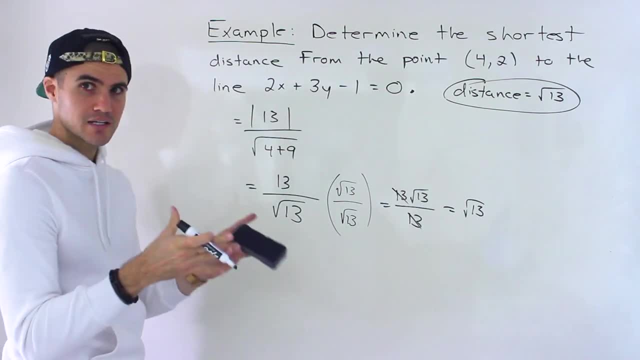 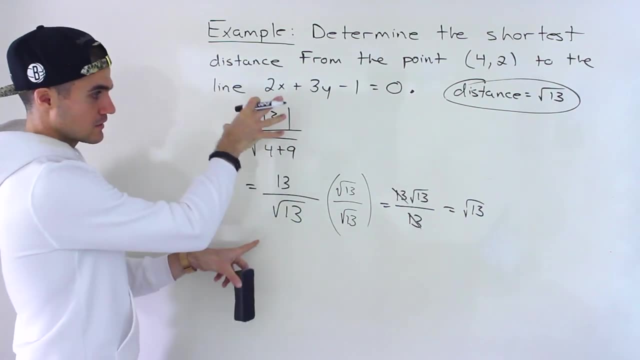 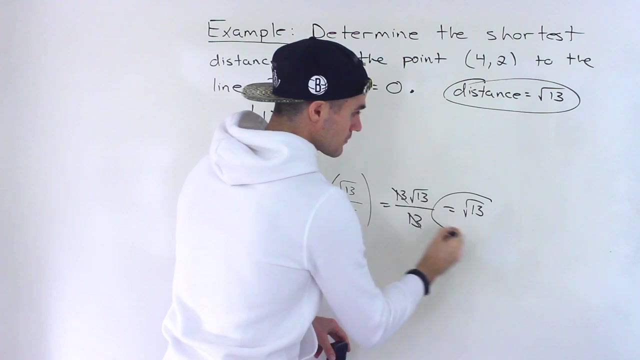 and we're just left with root 13 again. you may not be expected to know all this, okay? so when i'm doing all this, and if your teacher hasn't covered it, don't be intimidated. you may not even you need to use this formula that I'm showing you. I'm just showing you in case you want something.